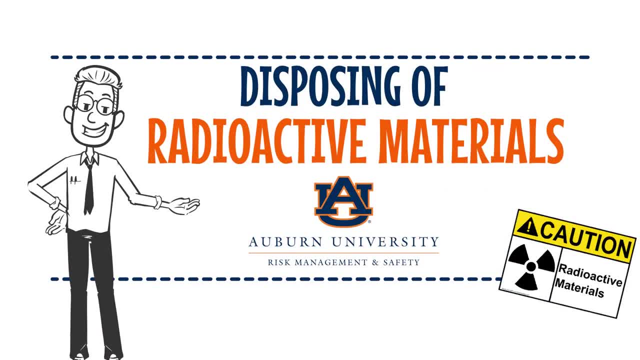 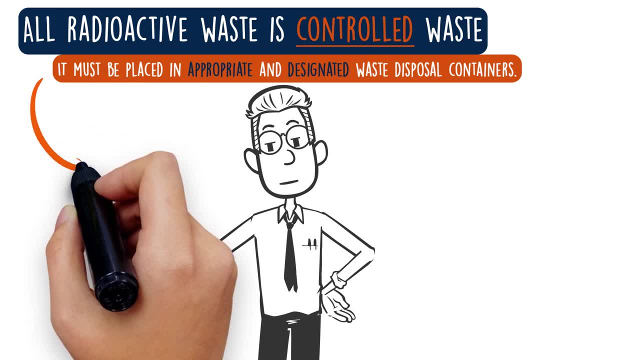 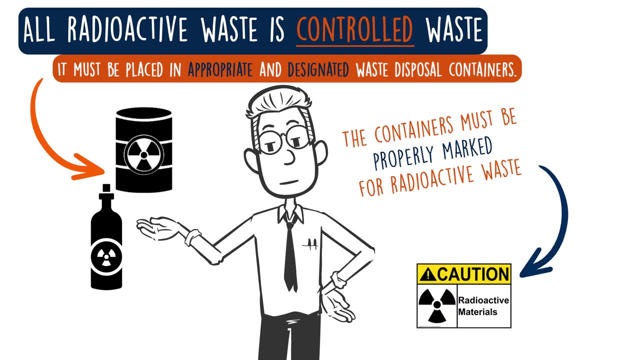 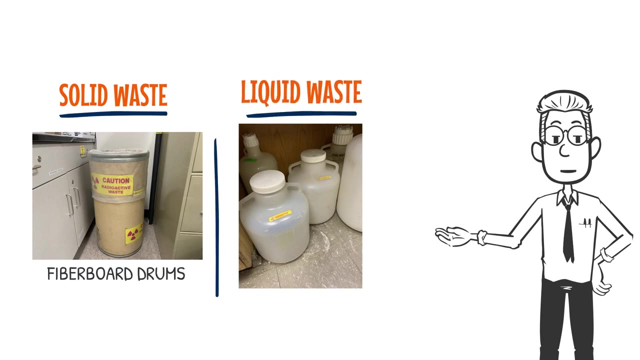 There are special requirements for disposing of radioactive materials. All radioactive waste is deemed controlled waste and must be placed in appropriate and designated waste disposal containers. The containers must be properly marked for radioactive waste. Auburn University uses fiberboard drums for solid radioactive waste and plastic jugs for liquid radioactive waste. The Radiation Safety Office can supply these. 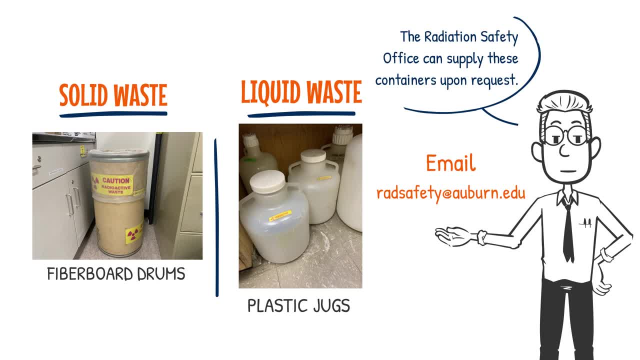 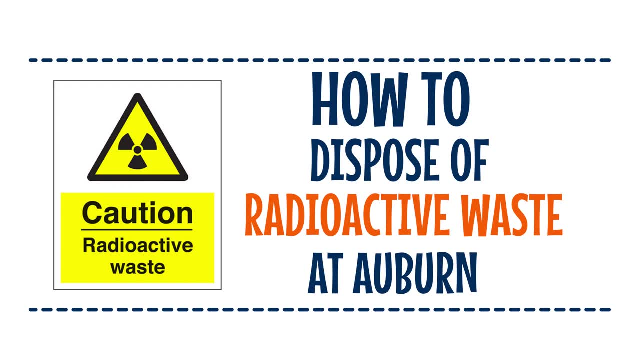 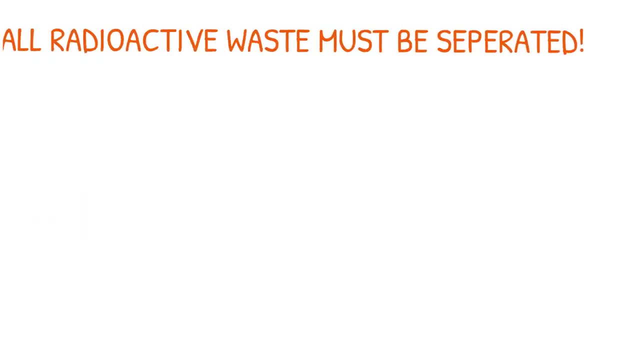 solid and liquid waste containers upon request. The disposal of radioactive waste, if not done properly, can be expensive for Auburn University. Here are a few simple steps that you can take to help with the disposal of radioactive waste. First, remember that all radioactive waste must be separated from non-radioactive waste. 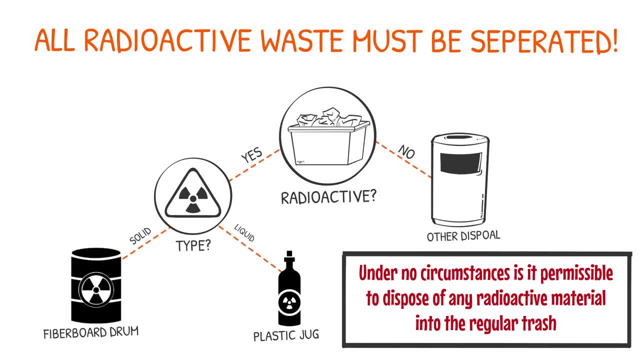 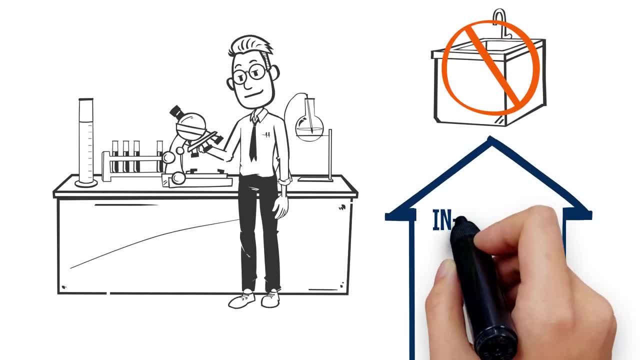 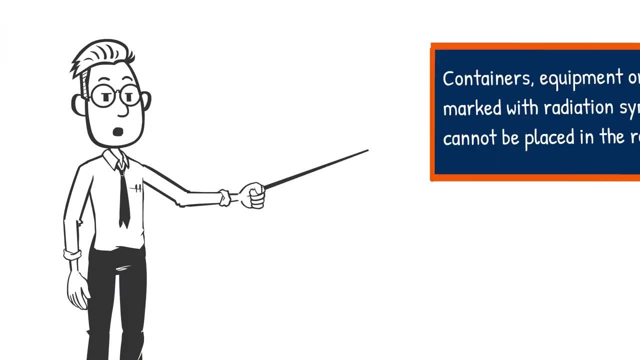 Under no circumstances is it permissible to dispose of any radioactive material into the regular trash. Second, in-lab sewer disposal of liquid waste is not allowed on Auburn University's campus. Third, no containers, equipment or supplies marked with radiation symbols and labels. 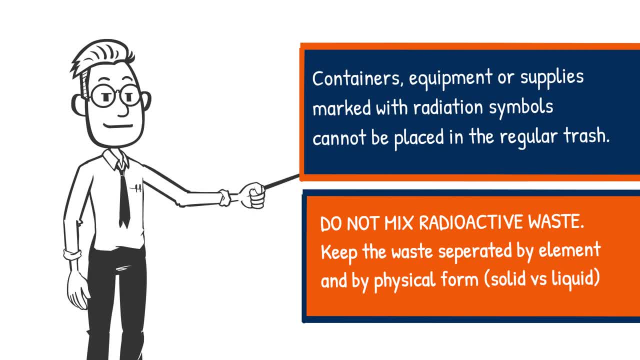 can be placed in the regular trash. Finally, radioactive waste should not be mixed. Keep the radioactive waste separate by radioactive element and physical form, such as solid or liquid. This allows for certain radioisotopes to be disposed of by decay in storage, In other words, allowing short-lived isotopes to decay to. 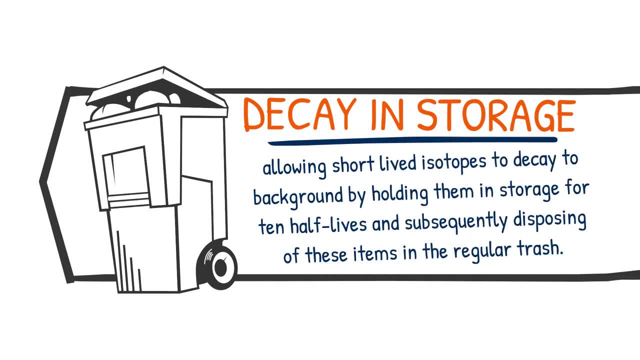 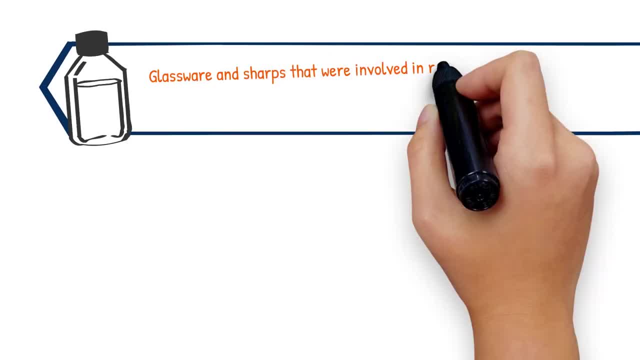 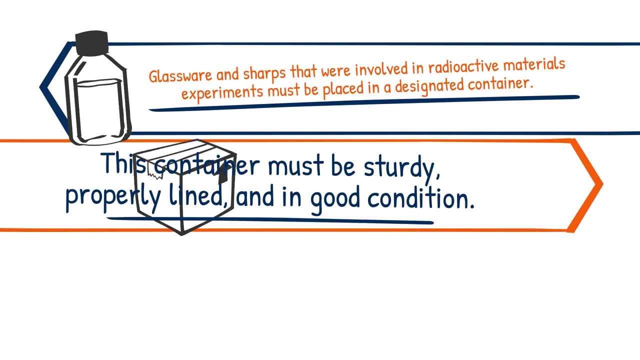 background by holding them in storage for 10 half-lives and subsequently disposing of these items in the regular trash. Glassware and sharps that were involved in radioactive materials- experiments must be placed in a designated container. This container must be sturdy, properly lined and in good condition. 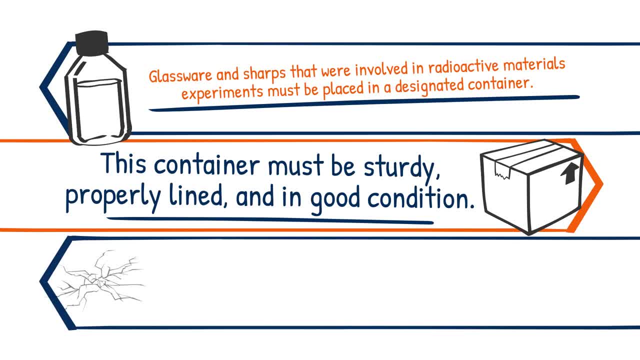 The container must be sturdy, properly lined and in good condition. Broken glass, wood and glass must be placed in a designated container. The container must be sturdy, properly lined and in good condition. The container must be sturdy, properly lined and in good condition. Broken glass, wood and glass must be placed in a designated container. The container must be sturdy, properly lined and in good condition. 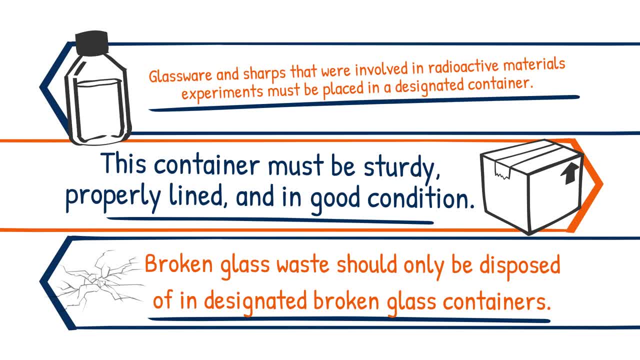 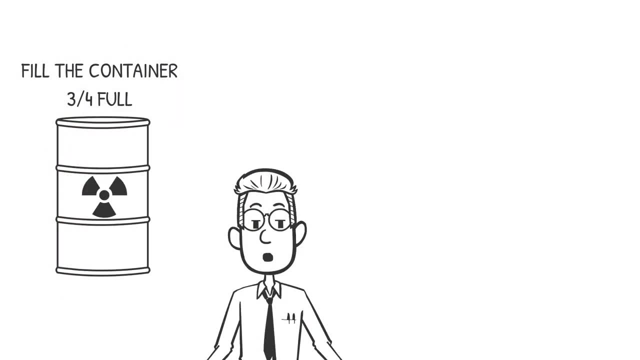 In designated broken glass containers. Radioactive materials, glassware and sharps containers should be labeled with caution, radiation or radioactive materials. When the solid waste fiberboard drum is slightly over 3 fourths full, it is ready to be picked up. Why 3 4ths? Because we do not want the